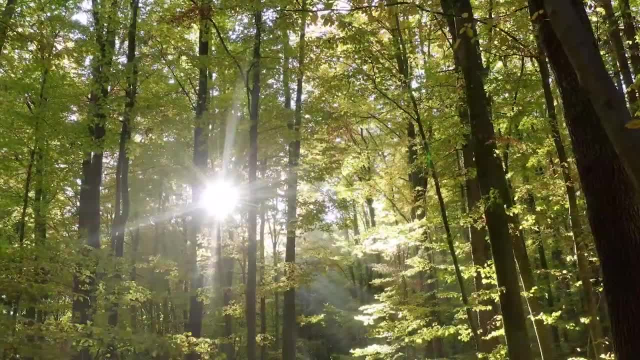 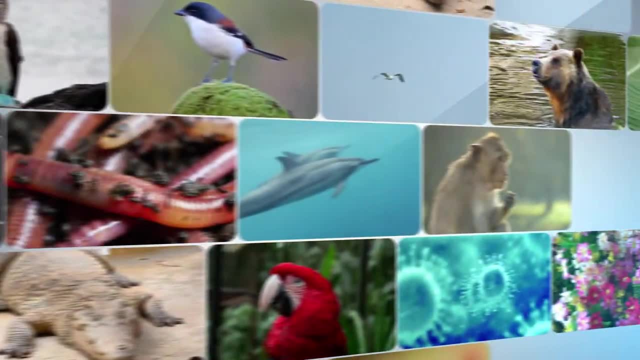 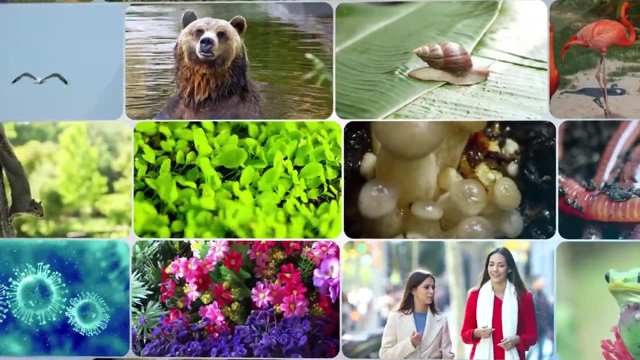 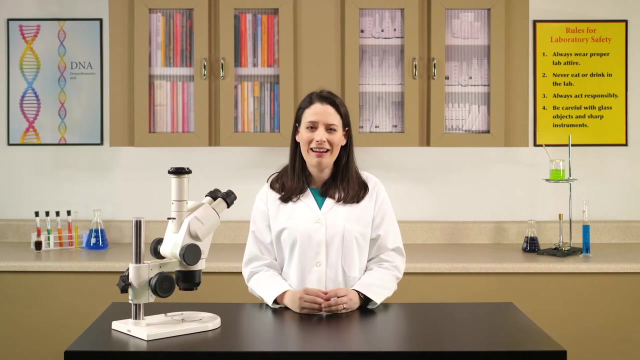 a forest with coniferous trees, a forest with coniferous trees with deciduous trees and a stream bank. each ecosystem contains billions of organisms: vertebrates, invertebrates, plants, fungi, bacteria and sometimes even humans, living together in balance. since it would be impossible to study all the 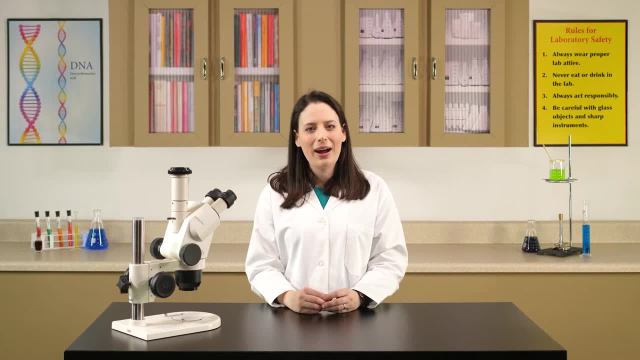 organisms in each ecosystem. we will limit our ecological survey to a small community of invertebrate organisms living within each ecosystem. the word community often refers to groups of people living in an area, but this word has a slightly different meaning to an ecologist, and ecological terms a 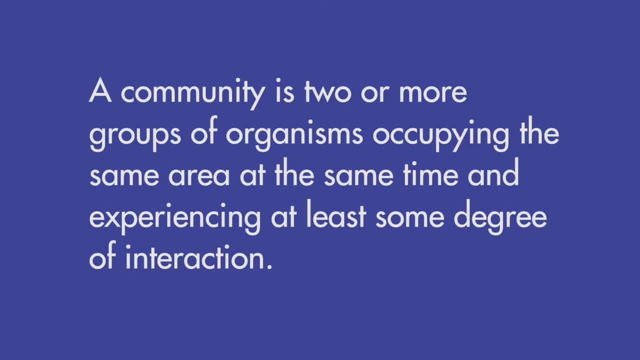 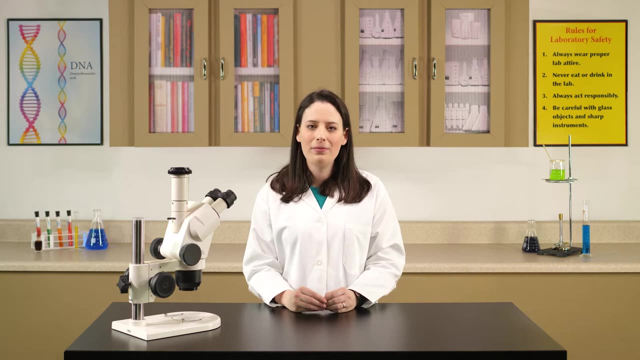 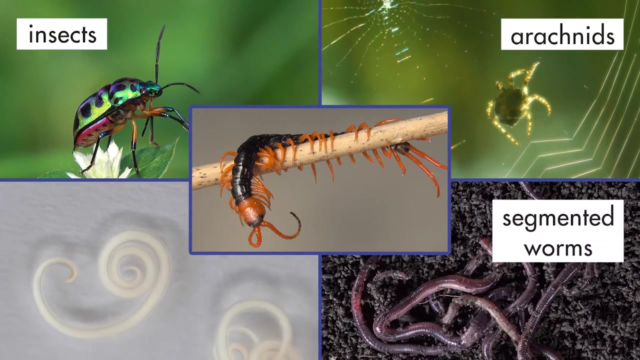 community is two or more groups of organisms occupying the same area at the same time and experiencing at least some degree of interaction. you for ease of study, we group the organisms of each soil sample into five categories of invertebrates, insects, arachnids, segmented worms, roundworms and myriapods. 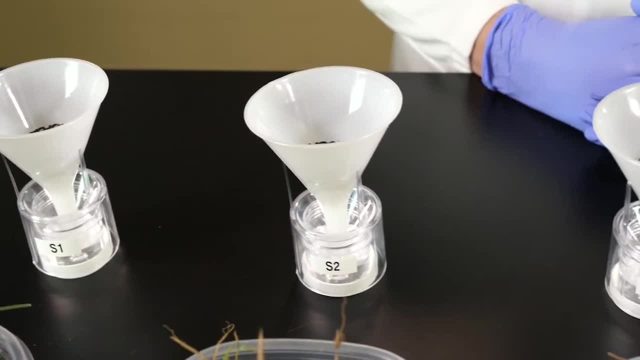 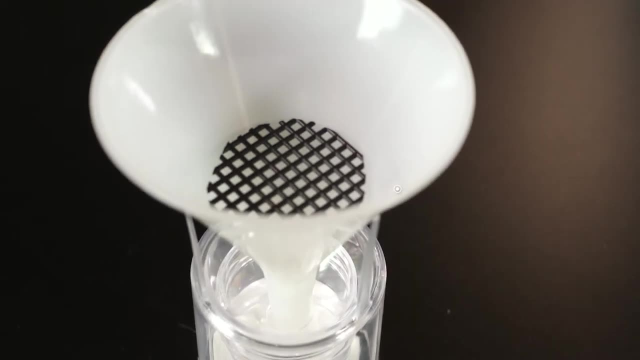 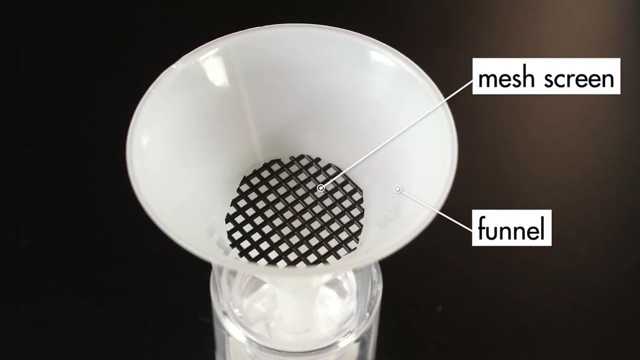 to collect the invertebrate organisms from a soil sample, we use a device known as a burlese trap. at the top of the burlese trap is a funnel with a mesh screen. the screen holds the soil sample in place, but it allows tiny organisms to. 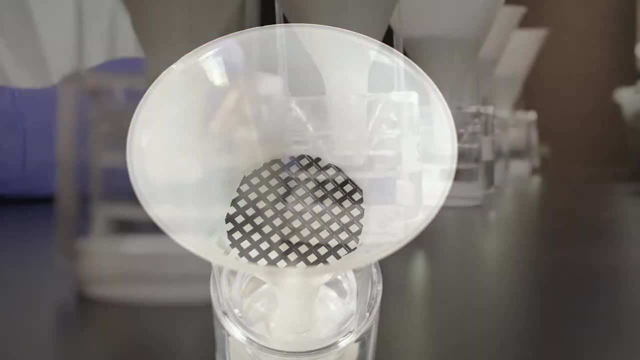 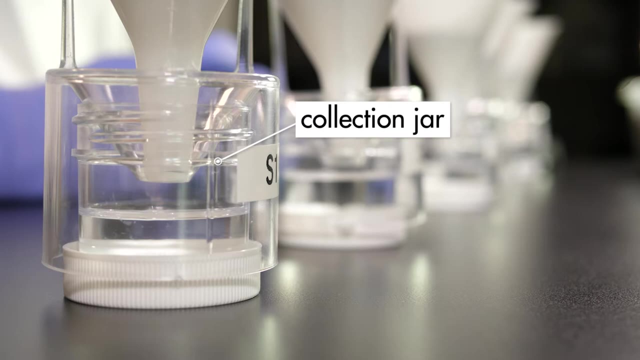 pass through organisms that pass through the screen drop into a small clear collection jar at the bottom of the trap. the collection jar contains 20 milliliters of isopropyl alcohol, which preserves the organisms so we can examine them later. we are ready to add soil from our first sample to the burlese. 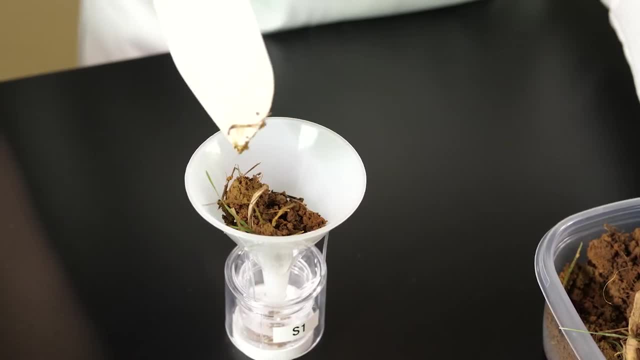 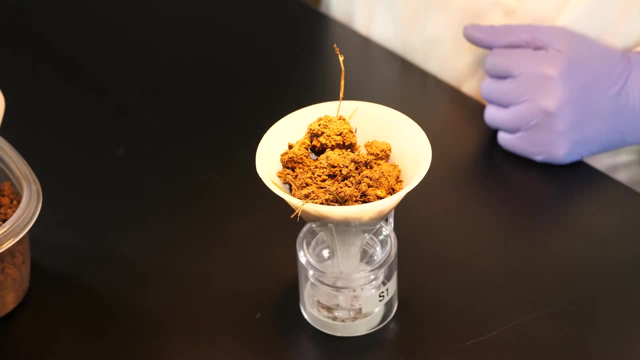 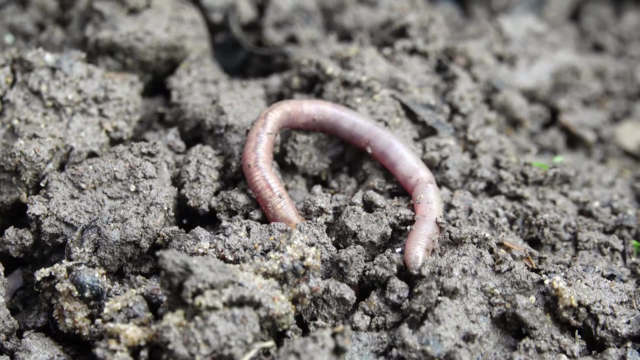 sample to the funnel. we must be careful not to force any soil through the screen. next we place the burlese trap under a lamp. the heat of the lamp dries out the soil, which forces the invertebrates to burrow deeper into the sample eventually. 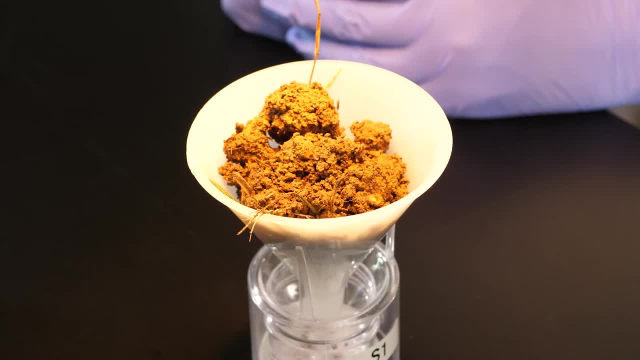 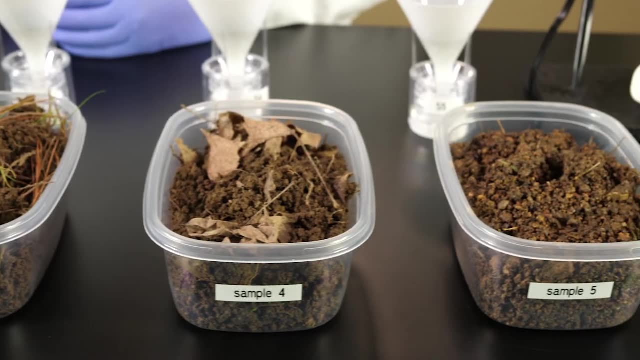 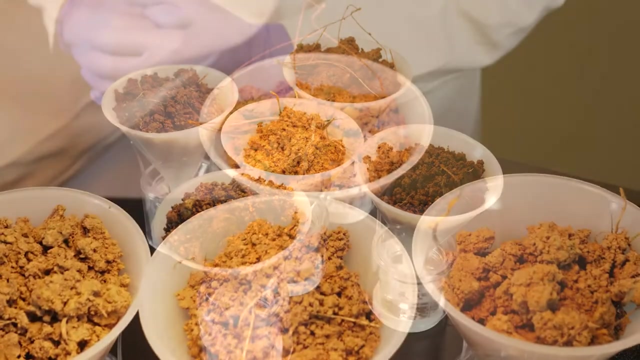 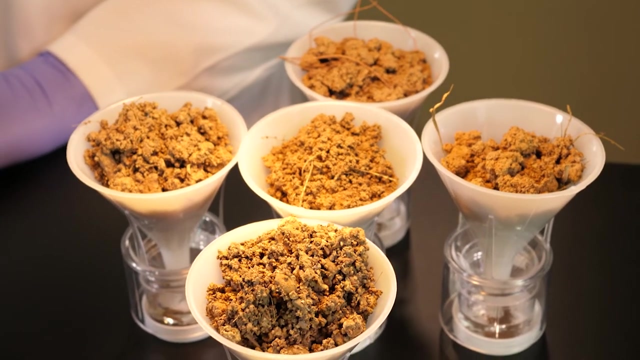 the invertebrates fall through the screen into the collection jar. we repeat the procedure with soil from the other four soil samples. we allow the burlese traps to sit under the lamp for three days. after three days we are ready to examine the results and determine biodiversity using two methods. 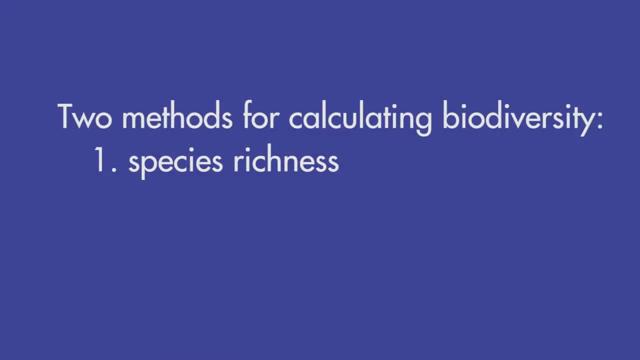 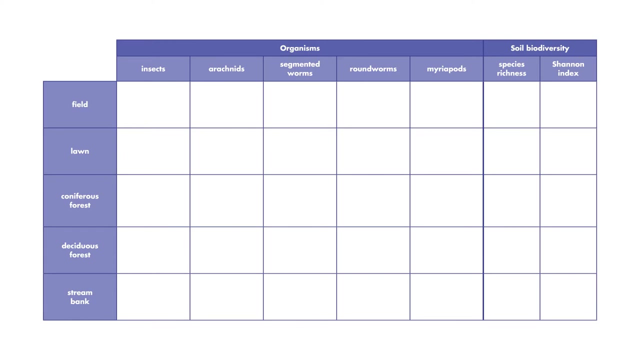 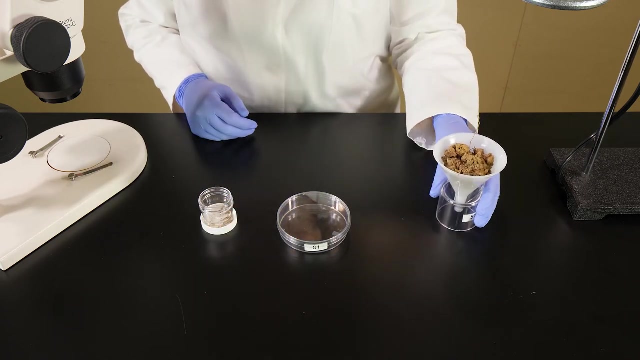 the first method produces a number called species richness. the second method produces a value called the Shannon index. we will record our observations and then we will record our observations. and then we will record our observations and a table so you can compare the results. first we will examine the organisms collected from the field ecosystem soil sample. since some 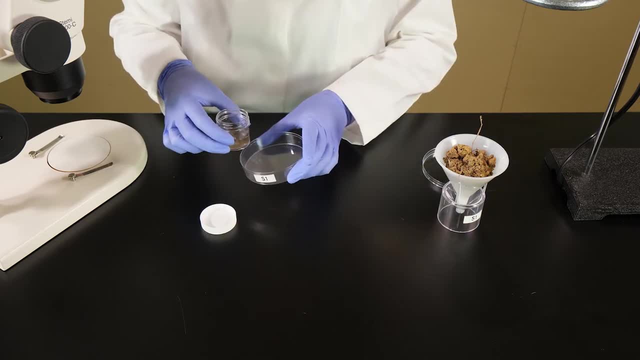 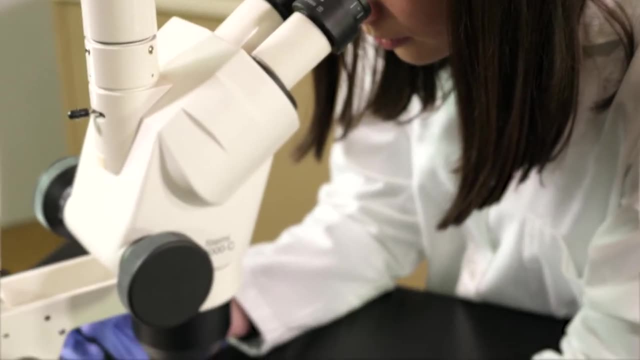 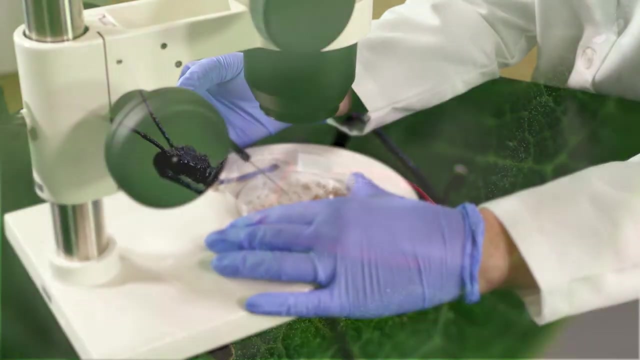 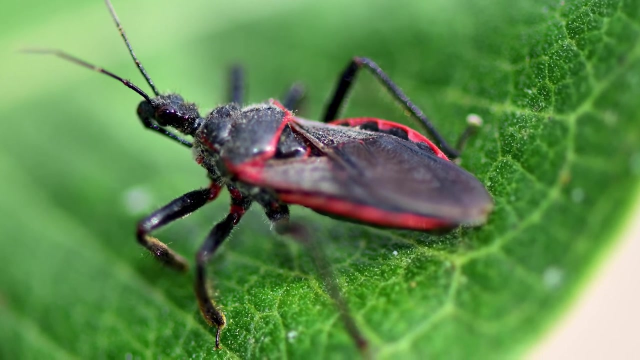 of the organisms are quite small. we will transfer them to a petri dish and examine them under the stereo microscope. while looking through the microscope, we move the members of each invertebrate category to a separate section of the petri dish. We move all ants, beetles and other insects to one section of the petri dish. 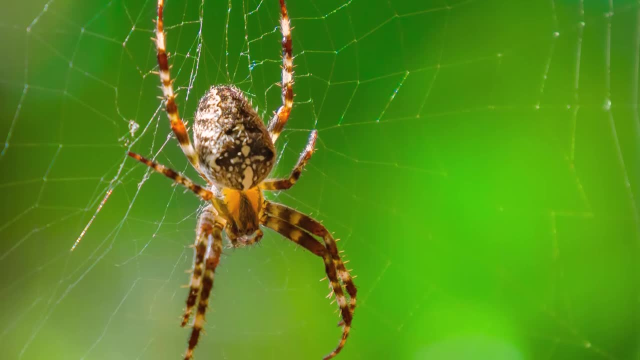 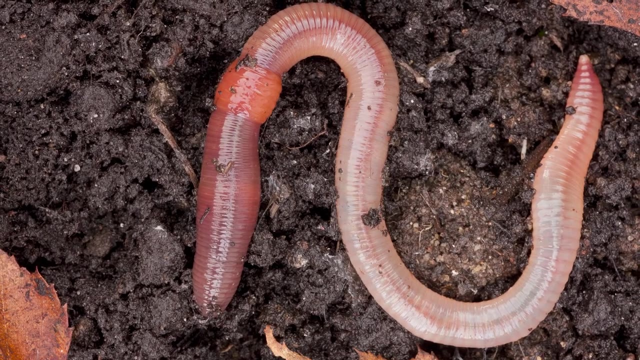 We move all spiders, ticks and other arachnids to another section. We move all earthworms, which are segmented worms, to another section. We move all roundworms, which are worms with smooth sides, to another section. 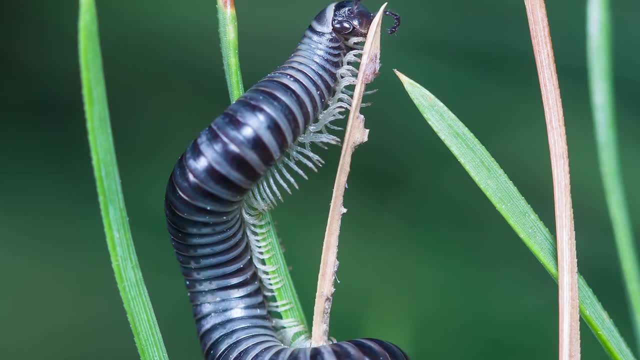 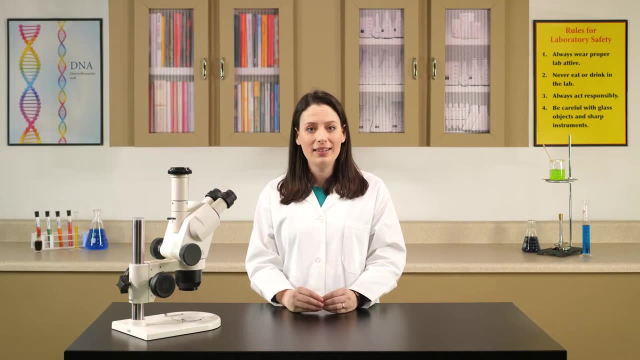 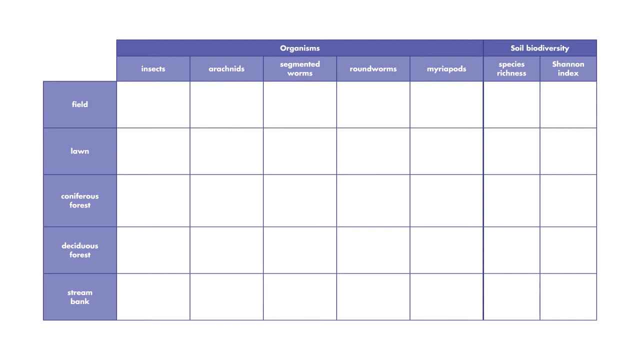 We move all centipedes and other myriapods to the remaining section. Now that the invertebrates have been sorted into categories, we count the number of organisms in each category and record these numbers in our table. We see that the soil sample from the field ecosystem has 8 insects. 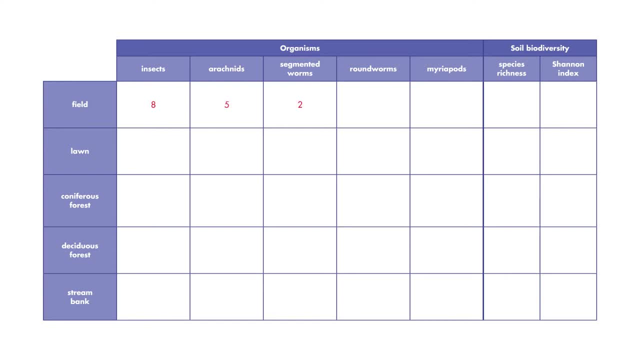 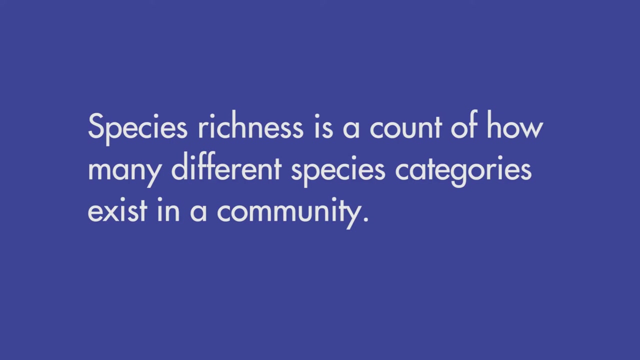 5 arachnids, 2 segmented worms, 12 roundworms and 3 myriapods. We follow the same procedure for the organisms found in each of the other soil samples and record those numbers on our table. Species richness is a count of how many different species categories exist in a community. 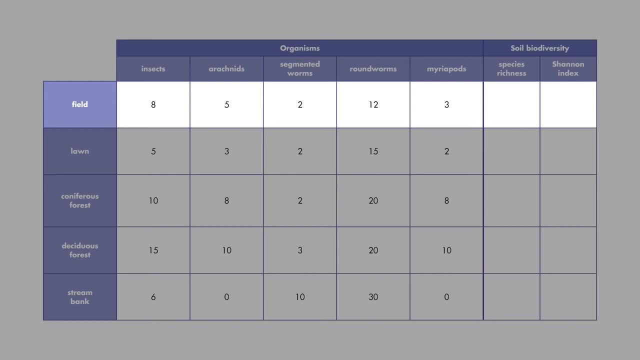 Since we found members of all 5 invertebrate categories in the field sample, the species richness of that soil sample is 4.. Notice that this value has been recorded in the species richness column on the table for the field sample, Since the same is true for the lawn sample and each of the forest samples. each of those soil samples also has a species richness of 5.. We did not find any arachnids or myriapods in the stream bank sample. We did find insects, segmented worms and roundworms. So this soil sample has a species richness of 3.. 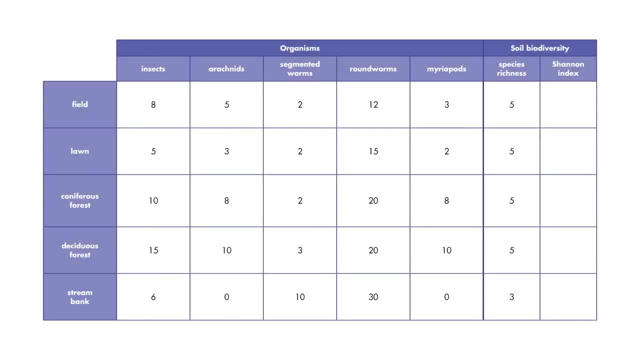 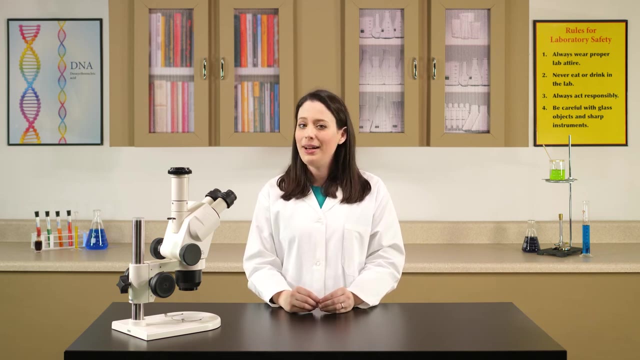 According to species richness, the field, lawn and forest communities have the same biodiversity. The stream bank has less biodiversity. Species richness tells us how many species categories exist in a sample, but it does not tell us how widely distributed those species are. Species richness tells us how many species categories exist in a sample, but it does not tell us how widely distributed those species are. Species richness tells us how many species categories exist in a sample, but it does not tell us how widely distributed those species are. 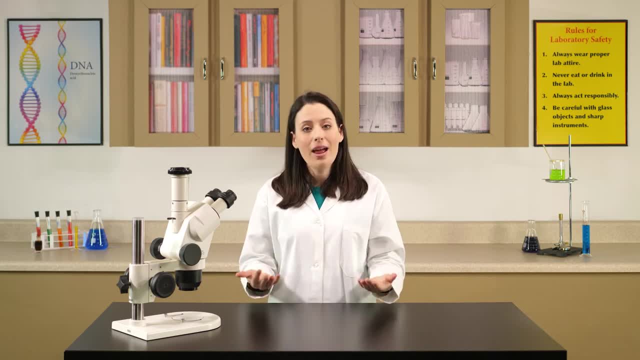 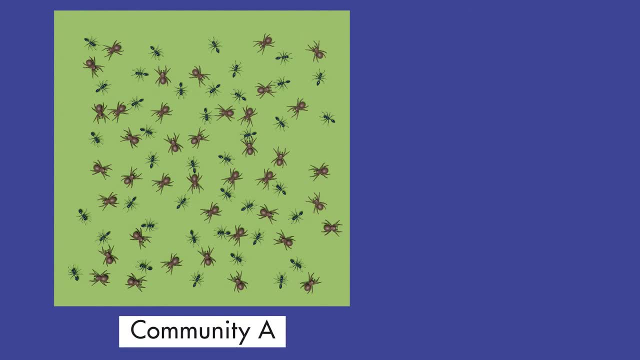 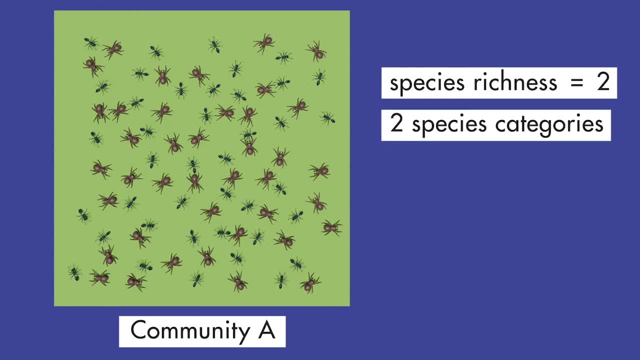 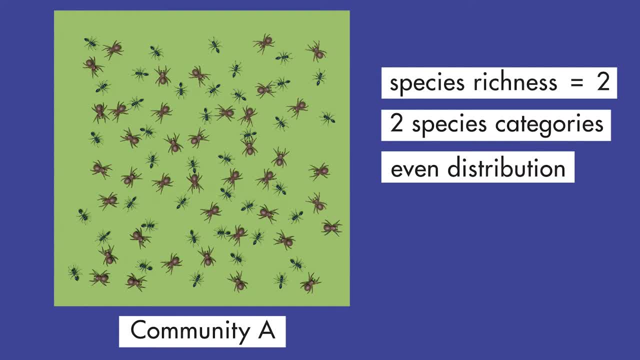 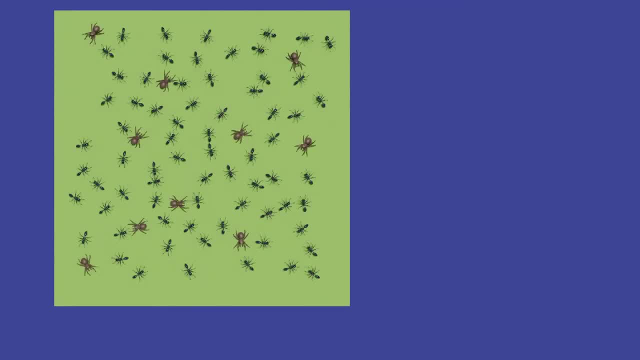 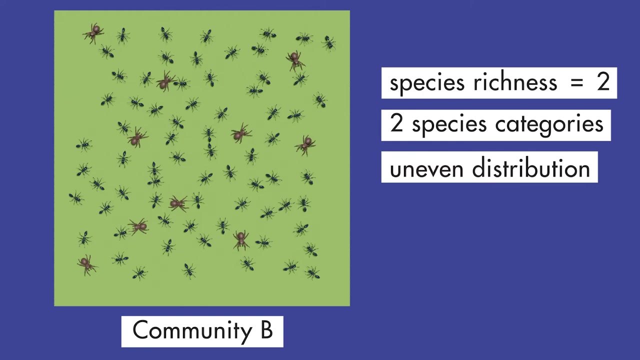 The distribution of organisms in Community A is even, but that fact is not reflected in the species richness number. In another example, Community B has 70 ants, but only 10 spiders. Community B also has a species richness of 2,, but the distribution of organisms in Community B is uneven. 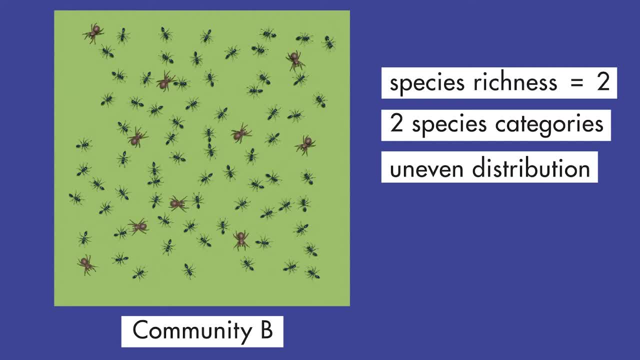 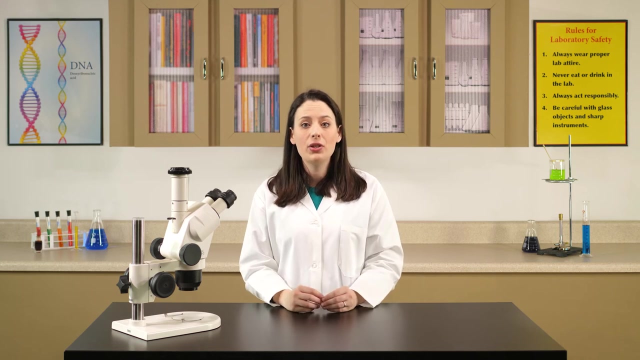 Both Communities, A and B, have the same number of species and the same species richness, but the biodiversity of each community is vastly different because of the distribution of the organisms. To indicate how many species categories exist in a community and how those organisms are distributed within the community: 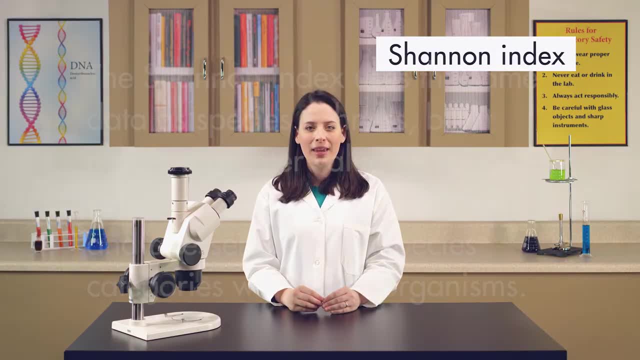 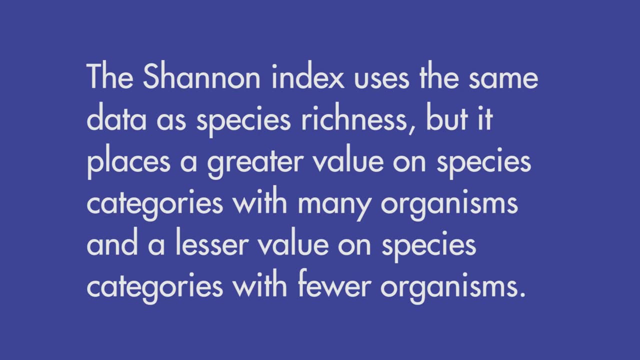 ecologists use the Shannon Index. The Shannon Index uses the same data that was used to determine species richness, but the data is calculated differently. A Shannon Index places a greater value on species categories with many organisms and a lesser value on species categories with fewer organisms. 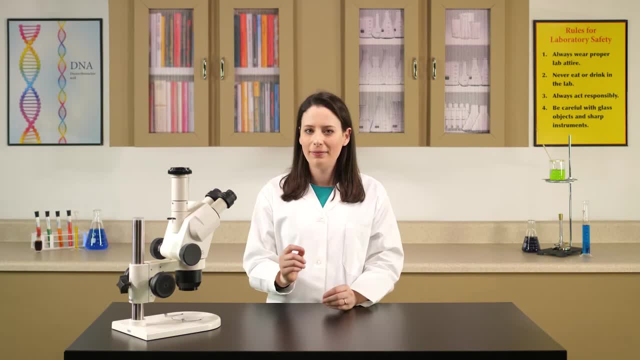 A Shannon Index ranges from 0 to 7.. If you recall, biodiversity is the variety of organisms and the number of species living in an area. If organisms in only one species category live in a community, then that community has no variety of organisms, so it has no biodiversity. 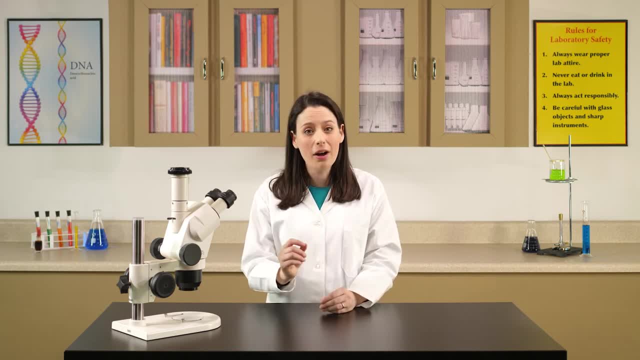 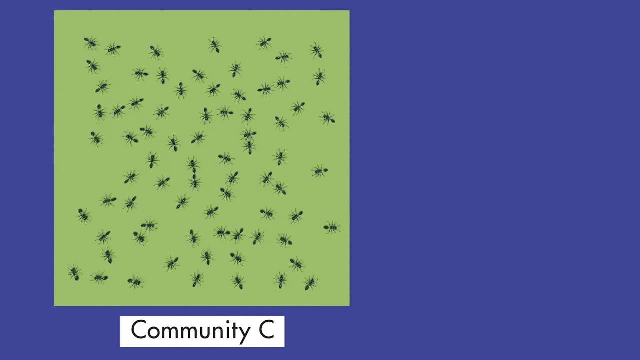 The Shannon Index of this community would be 0.. In this example, Community C has 76 organisms. Since all 76 organisms are in one species category, the species richness is 0.. The Shannon Index for Community C is 1,, but the Shannon Index for Community C is 0. 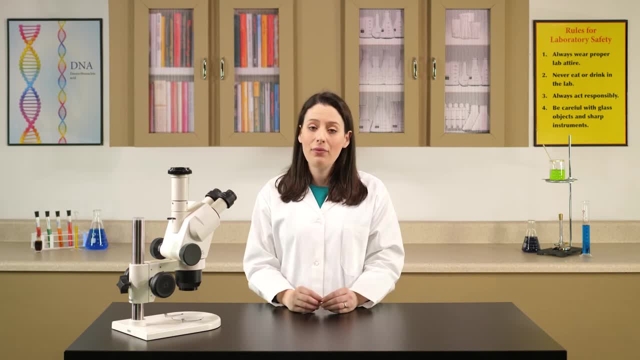 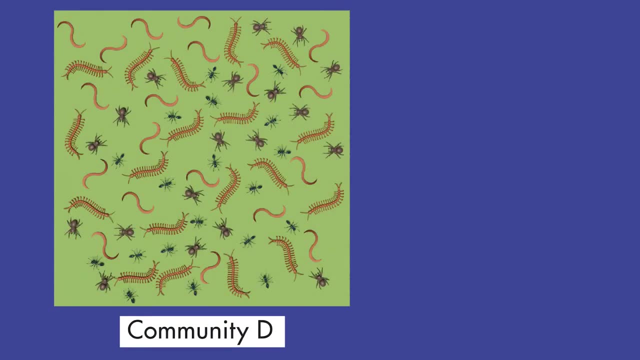 A community with organisms evenly distributed among several species categories would have a higher Shannon Index. In this example, Community D also has 76 organisms, but they are evenly distributed among four species categories. Community D has a species richness of 4,, but they are equally distributed among four species categories. 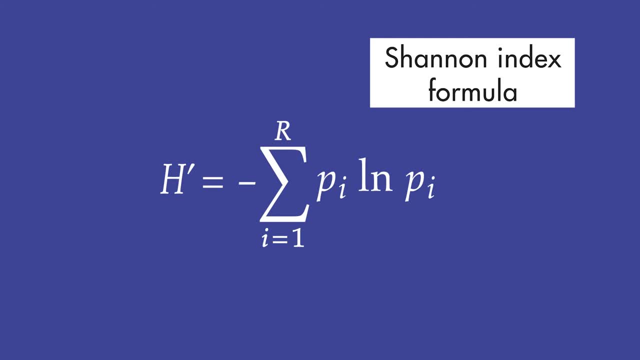 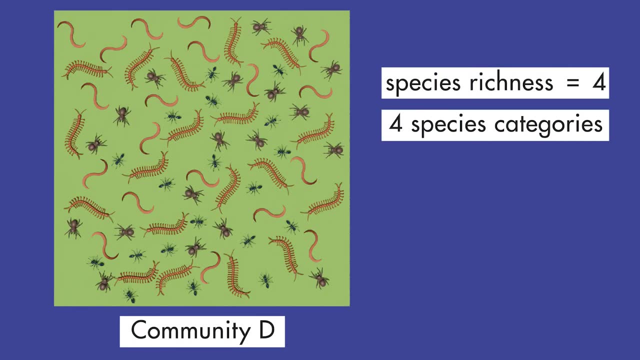 Determining a Shannon Index requires some complex mathematics, so we will not go through the steps of calculating the Shannon Index at this time. Instead, we will provide you with the Shannon Index values for this experiment: The Shannon Index values and the species richness numbers. 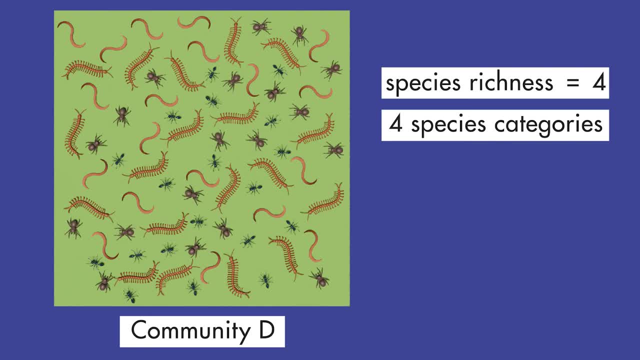 indicate the biodiversity and the potential for supporting life. The Shannon Index for Community D is 1,, but they are equally distributed among four species categories. The Shannon Index for Community E is 1.. The Shannon Index for Community H is 1.. And the Shannon Index for Community B is 1.. 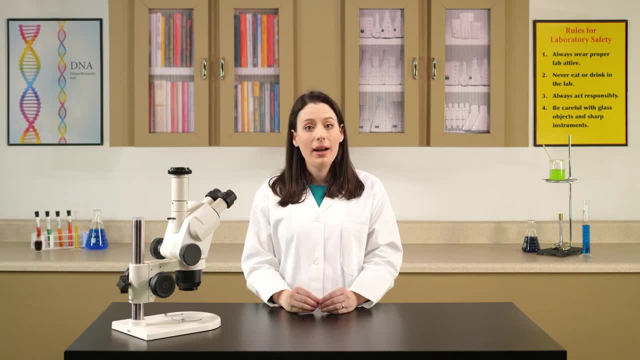 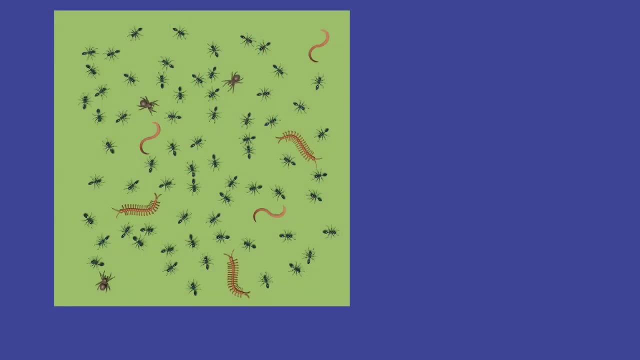 The Shannon Index for Community H is 1.. The Shannon Index for Community C is 1.. A community with the same species richness but with organisms less evenly distributed would have a lower Shannon Index. In this example, Community E also has 76 organisms in four species categories.